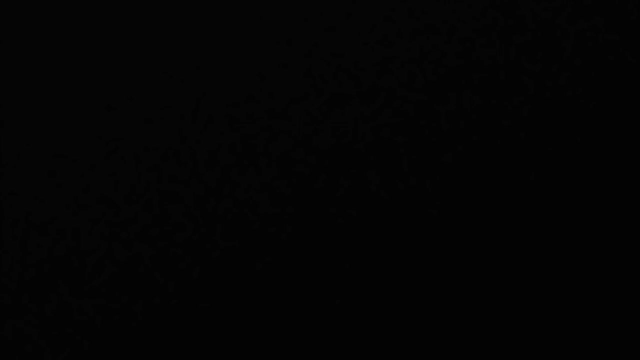 So now that we've spent some time thinking about what a differential equation is, and even visualizing solutions to a differential equation using things like slope fields, let's start seeing if we can actually solve differential equations And, as we'll see, different types of differential equations. 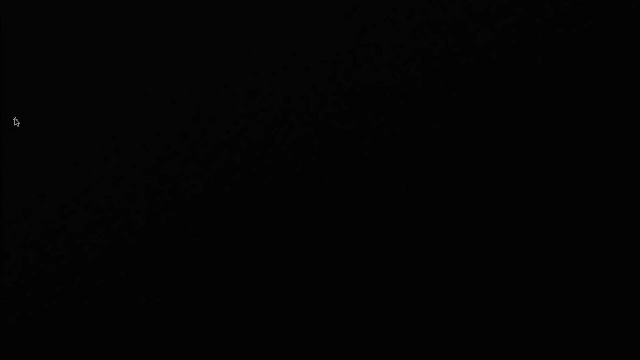 might require different techniques, and some of them we might not be able to solve at all using analytic techniques. We'd have to resort to numeric techniques to estimate the solutions. But let's go to what I would argue is the simplest form of differential equation to solve. 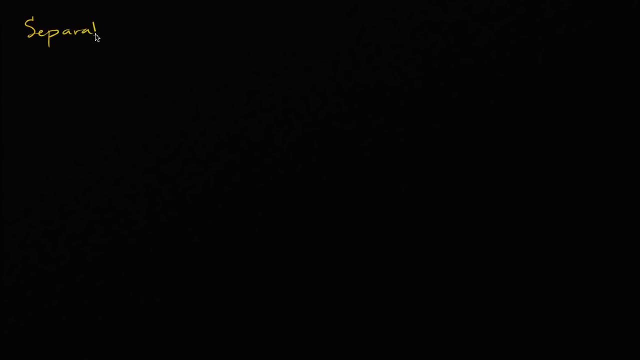 and that's what's called a separable differential equation, And we will see in a second why it is called a separable differential equation. So let's say that we have the derivative of y with respect to x is equal to negative x over ye to the x squared. 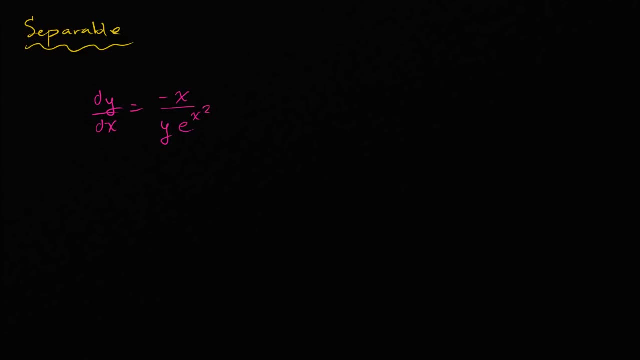 So we have this differential equation and we want to find the particular solution that goes through the point zero, comma one, And I encourage you to pause this video and I'll give you a hint, If you can, on one side of this equation. 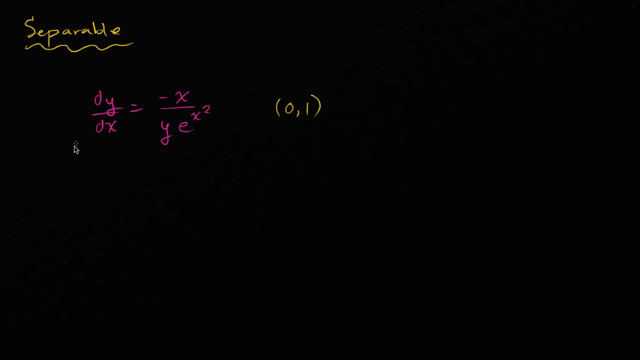 through algebra: separate out the y's and the dy's and on the other side have all the x's and dx's and then integrate. perhaps you can find the particular solution to this differential equation that contains this point. Now, if you can't do it, don't worry. 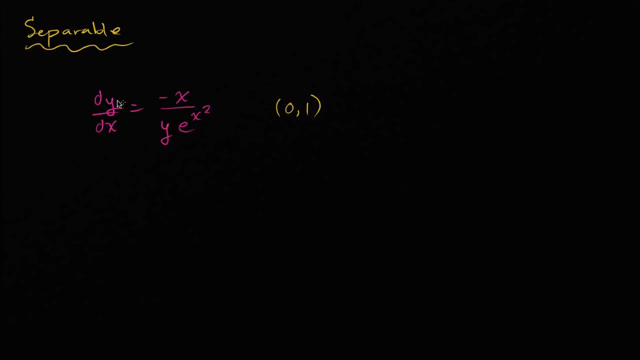 because we're about to work through it. Subtitles by the Amaraorg community. So, as I said, let's use a little bit of algebra to get all the y's and dy's on one side and all the x's and dx's on the other side. 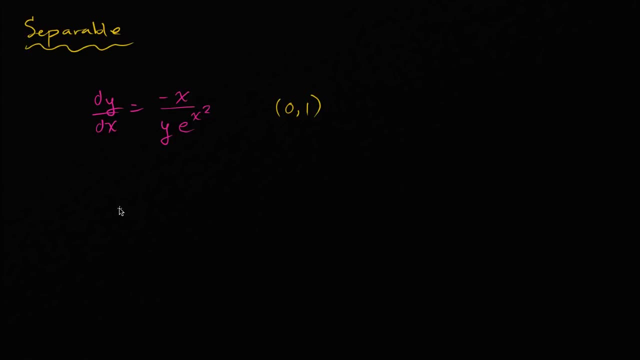 So one way if I want. let's say I want to get all the y's and dy's on the left-hand side and all the x's and dx's on the right-hand side. Well, I can multiply both sides. times y. 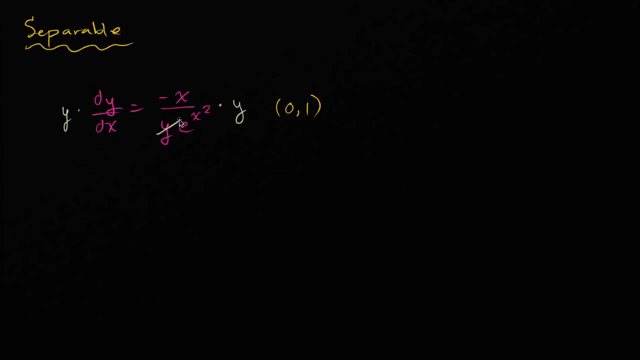 So I can multiply both sides times y. That has the effect of putting the y's on the left-hand side And then I can multiply both sides times dx. I can multiply both sides times y. Subtitles by the Amaraorg community. And we kind of treat, you can treat these differentials. 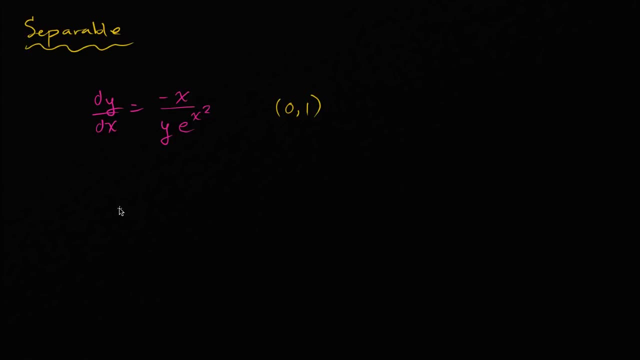 So one way if I want. let's say I want to get all the y's and dy's on the left-hand side and all the x's and dx's on the right-hand side. Well, I can multiply both sides. times y. 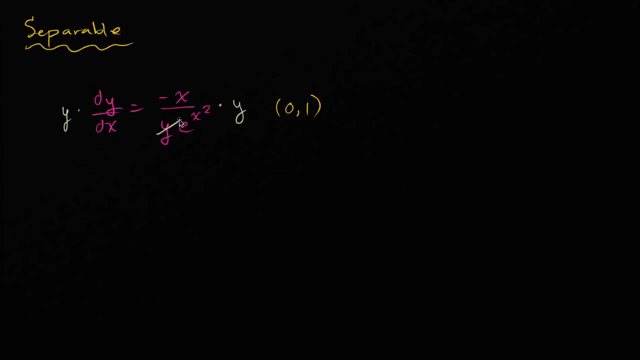 So I can multiply both sides times y. That has the effect of putting the y's on the left-hand side And then I can multiply both sides times dx. I can multiply both sides times y. Subtitles by the Amaraorg community. And we kind of treat, you can treat these differentials. 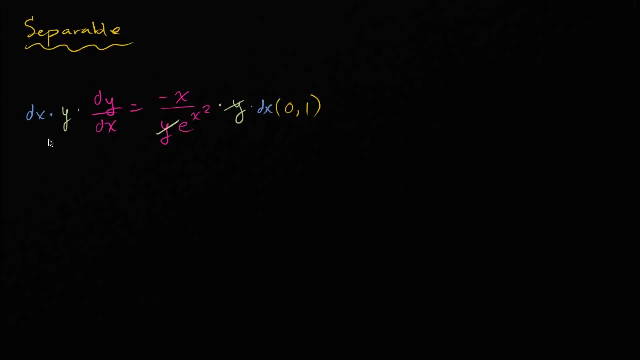 as you would treat a variable when you're manipulating it to essentially separate out the variables, And so this will cancel with that, And so we are left with. we are left with y dy. y dy is equal to negative x, and actually let me write it this way: 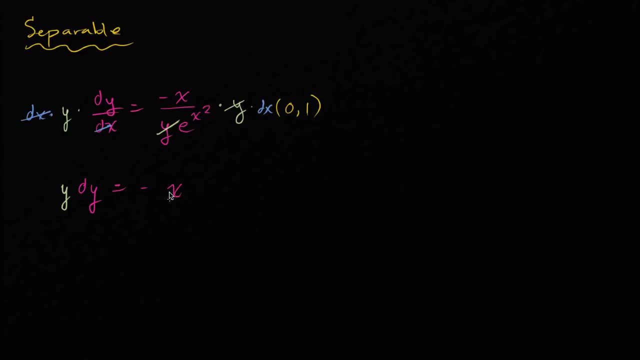 Let me write it as negative xe. actually I might a little more space. So negative xe to the negative: x squared, dx, dx. Now why is this interesting? Because we could integrate both sides. And now this also highlights why we call this separable. 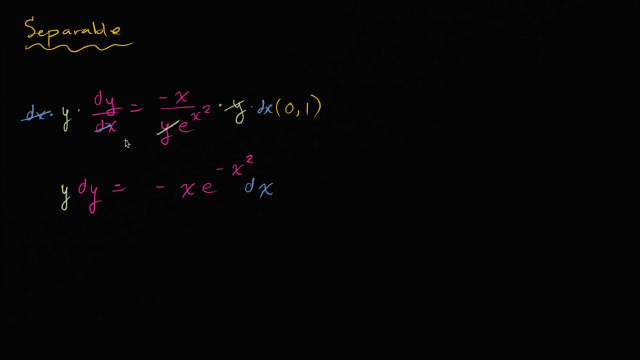 You won't be able to do this with every differential equation. You won't be able to algebraically separate the y's and dy's on one side and the x's and dx's on the other side. But this one we were able to. 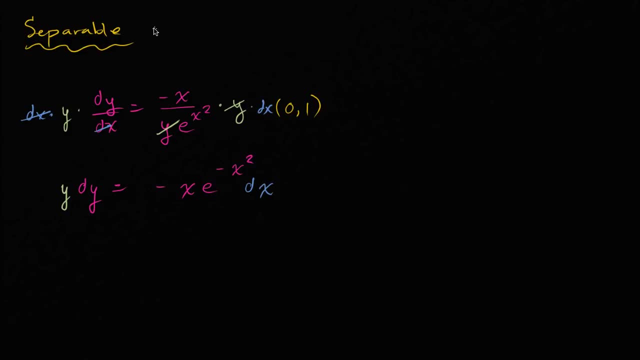 And so that's why this is called a separable differential equation, And it's usually the first technique that you should try. Hey, can I separate the y's and the x's? And, as I said, this is not going to be true. 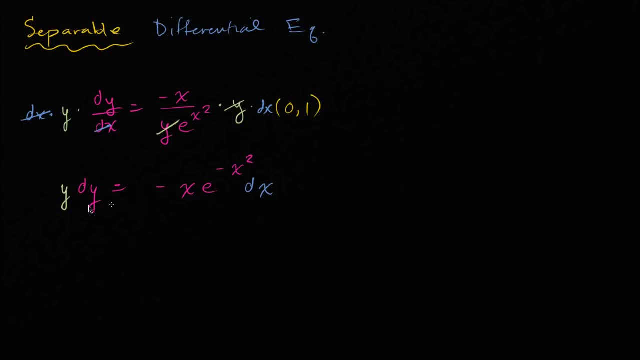 of many, if not most, differential equations. But now that we did this, we can integrate both sides. So let's do that. So I'll find a nice color to integrate with. So I'm going to integrate both sides. Now, if you integrate the left-hand side, what do you get? 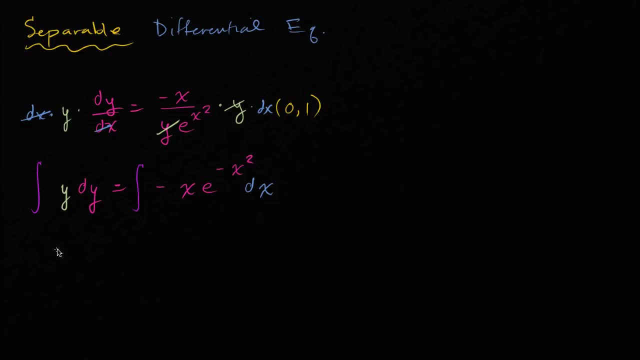 You get and remember we're integrating with respect to y here. So this is going to be y squared over two And we could put some constant there. I could call that plus c one And if you're integrating now, that's going to be equal to. 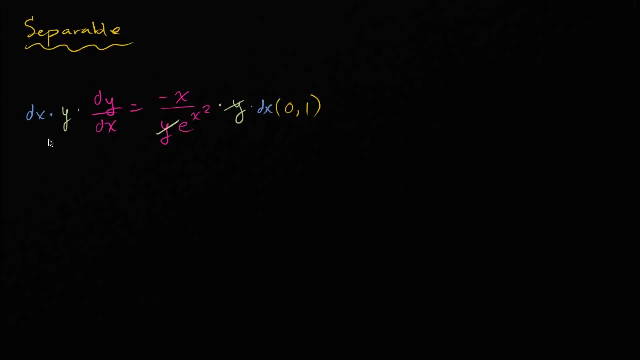 as you would treat a variable when you're manipulating it to essentially separate out the variables, And so this will cancel with that, And so we are left with. we are left with y dy. y dy is equal to negative x, and actually let me write it this way: 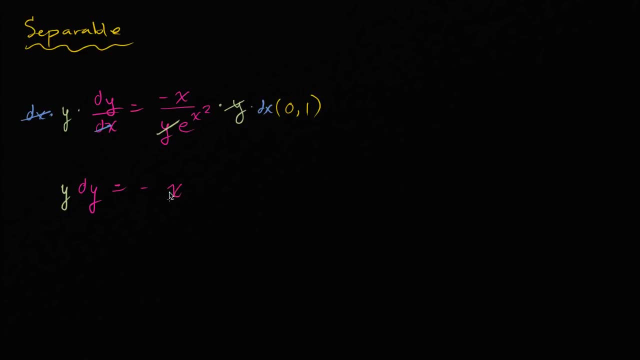 Let me write it as negative x e. actually I might a little more space. So negative x e to the negative x, squared dx, Dx. Now why is this interesting? Because we can integrate both sides. And now this also highlights why we call this separable. 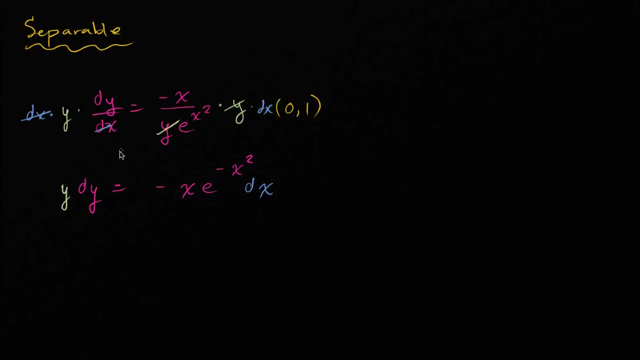 You won't be able to do this with every differential equation. You won't be able to algebraically separate the y's and dy's on one side and the x's and dx's on the other side. But this one we were able to. 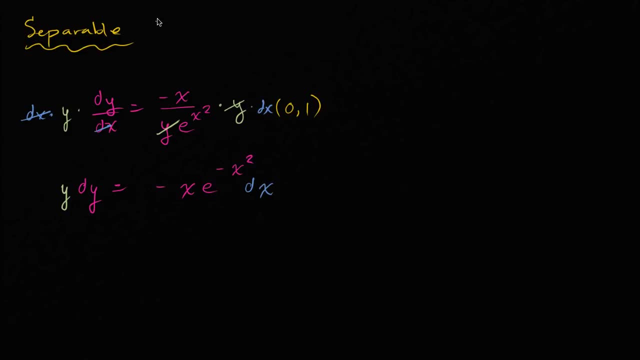 And so that's why this is called a separable differential equation, Differential differential equation, And it's usually the first technique that you should try. Hey, can I separate the y's and the x's? And, as I said, this is not going to be true. 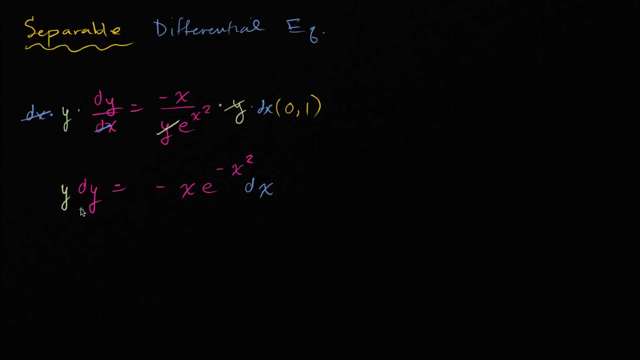 of many, if not most, differential equations. But now that we did this, we can integrate both sides. So we can integrate both sides. So let's do that, So I'll find a nice color to integrate with. So I'm going to integrate. integrate both sides. 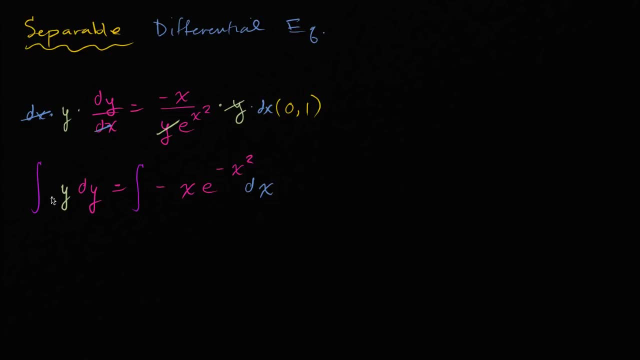 Now, if you integrate the left hand side, what do you get? You get- and remember, we're integrating with respect to y here. So this is going to be y squared over two, And we could put some constant there. I could call that plus c one. 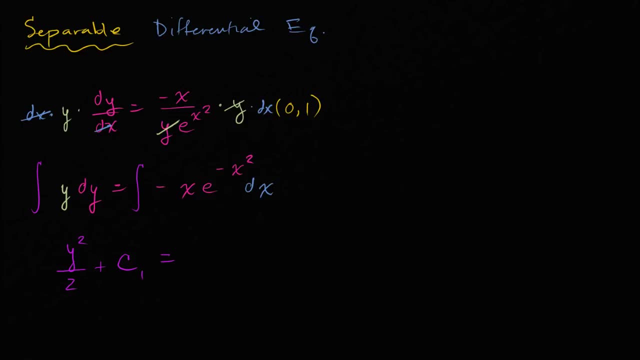 And if you're integrating now, that's going to be equal to now the right hand side. we're integrating with respect to x And let's see, you could do u substitution or you could recognize that. look, the derivative of negative x squared. 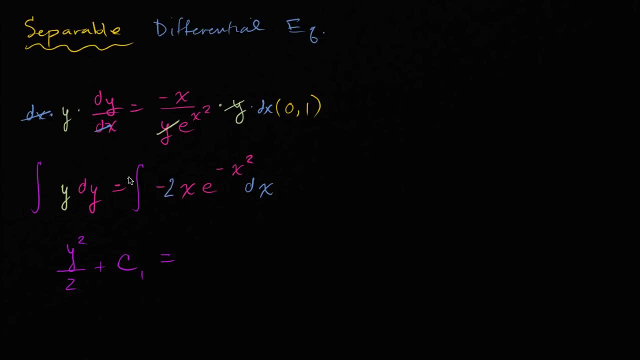 is going to be negative two x. So if that was a two there, and if you don't want to change the value of the integral, you put the one half right over there. And so now you could either do u substitution explicitly or you could do it in your head. 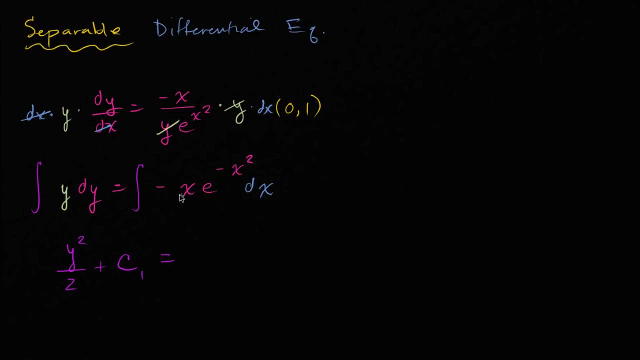 now the right-hand side we're integrating with respect to x. And let's see, You could do u-substitution or you could recognize that. look, the derivative of negative x squared is going to be negative 2x. So if that was a two there and if you don't want to change, 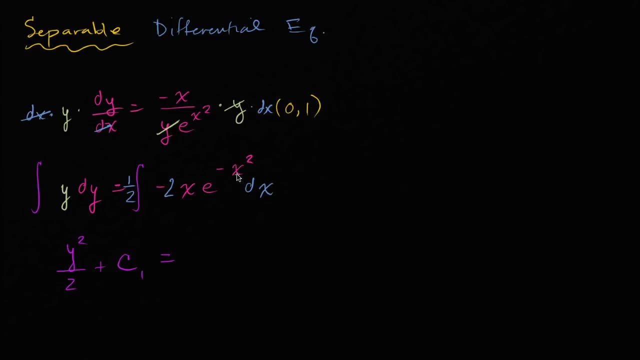 the value of the integral. you put the 1 half right over there, And so now you could either do u-substitution explicitly, or you could do it in your head, Or you set u is equal to negative x squared, And then du will be negative 2x dx. 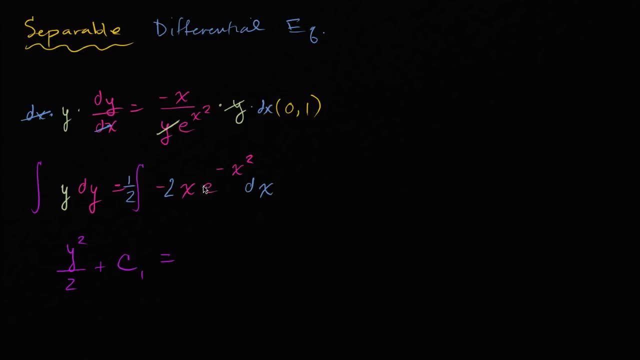 Or you can kind of do this in your head at this point. So I have something and it's derivative, So I really could just integrate with respect to that something, with respect to that u. So this is going to be 1 half this, 1 half right over here. 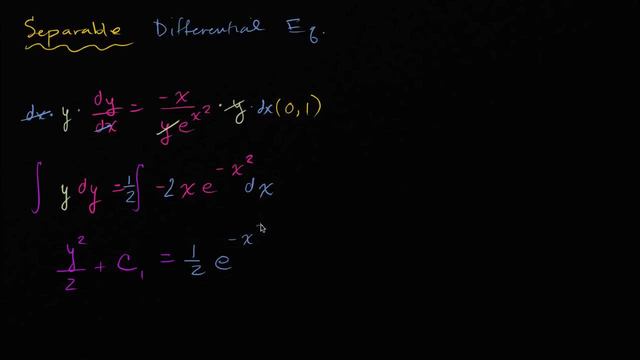 The anti-derivative of this is e to the negative x squared. And then of course I might have some other constant. I'll just call that c two. And once again- if this part over here, what I just did, seemed strange, the u-substitution. 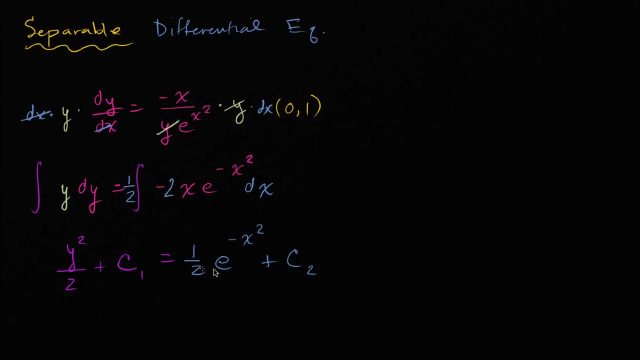 you might want to review that piece. Now, what can I do here? Well, I have a constant on the left-hand side. It's an arbitrary constant. We don't know what it is. I haven't used this initial condition yet. we could call it. 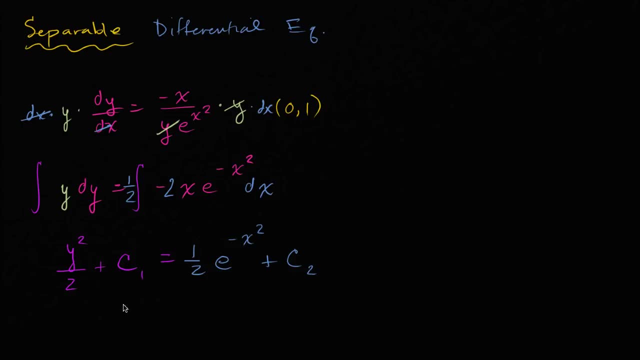 So let me just subtract c one from both sides. So if I just subtract c one from both sides, I have an arbitrary. so this is going to cancel, And I have c two, sorry, let me. so this is c one. 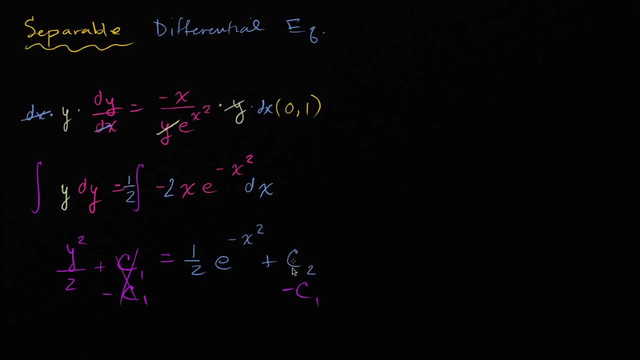 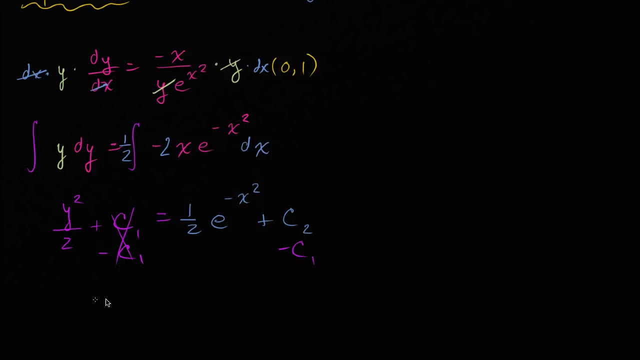 So these are going to cancel, And c two minus c one. these are both constants, arbitrary constants. We don't know what they are yet, And so we could just do that. We could just rewrite this as on the left-hand side. 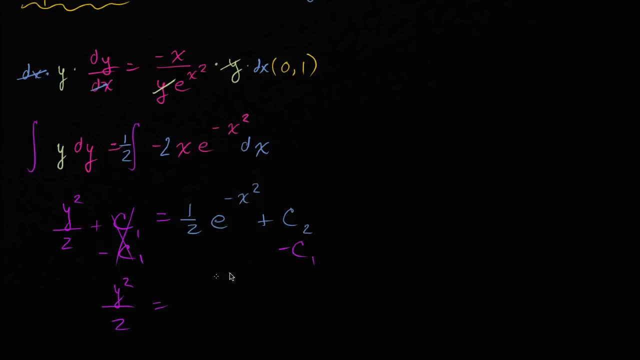 we have y squared over two is equal to on the right-hand side. I'll write one half e. let me write that in blue, just because I wrote it in blue before. One half, one half e to the negative x squared. 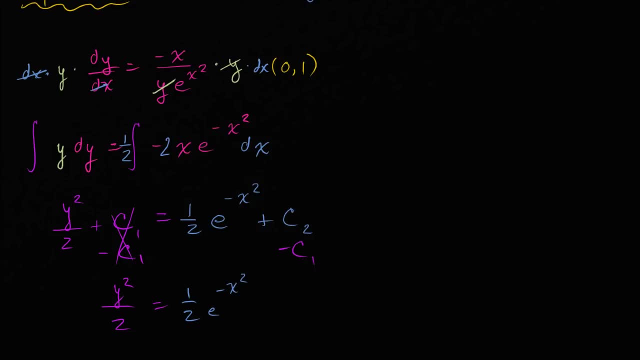 And I'll just say c two minus c one. let's just call that c. So if you take the sum of those two things, let's just call that c. And so now this is kind of a general solution. We don't know what this constant is. 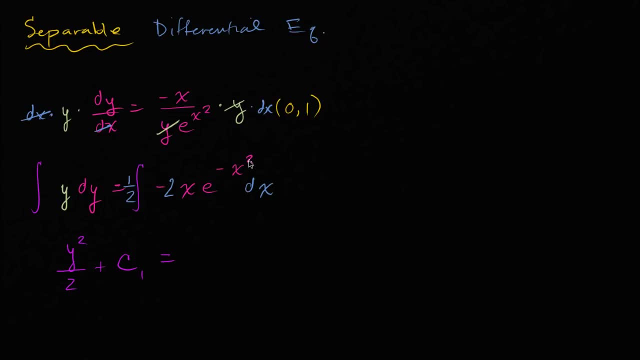 or you set u is equal to negative x squared, and then du will be negative two x dx, Or you can kind of do this in your head at this point. So I have, I have something and it's derivative, so I really could just integrate with respect to that something. 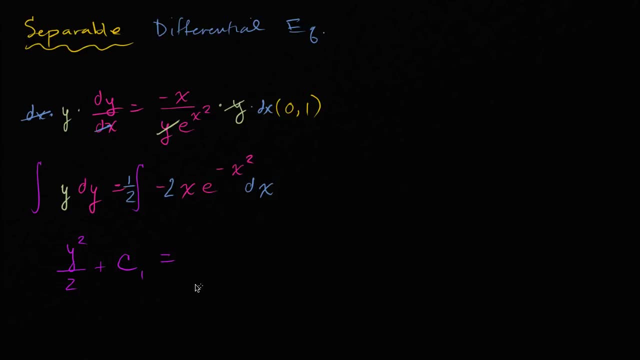 with respect to that u. So this is going to be, this is going to be one half this, one half right over here. The anti-derivative of this is e to the negative, x squared, And then, of course, I might have some other constant. 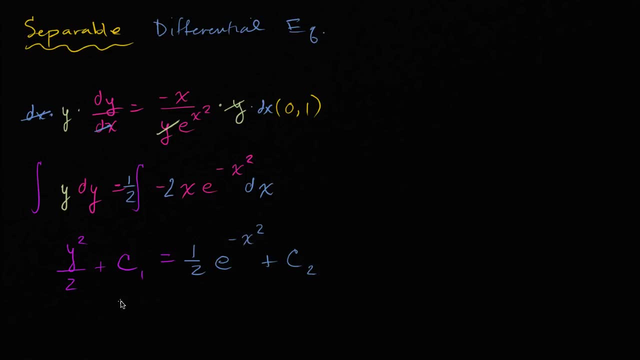 I'll just call that c. two, And once again, if this part over here, what I just did, seemed strange, the u substitution, you might want to remember that. You might want to review that piece Now, what can I do here? 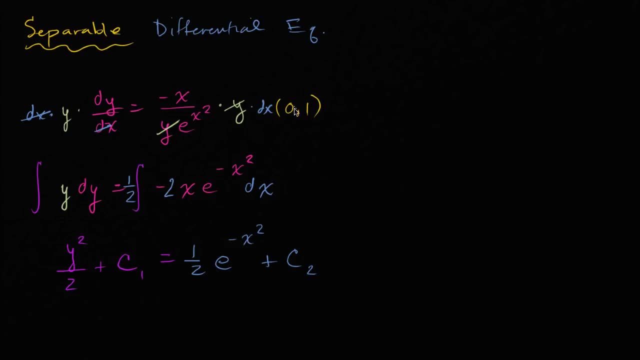 Well, I have a constant on the left-hand side. It's an arbitrary constant. We don't know what it is. I haven't used this initial condition yet we could call it, So let me just subtract c one from both sides. 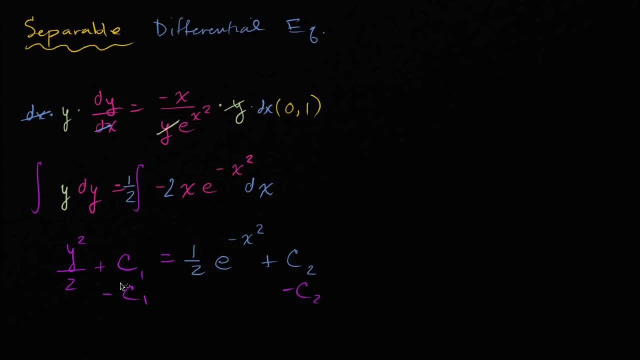 So if I just subtract c one from both sides, I have an arbitrary, so this is going to cancel, And I have c two. sorry, let me. so this is c one, So these are going to cancel. And c two minus c one, these are both constants. 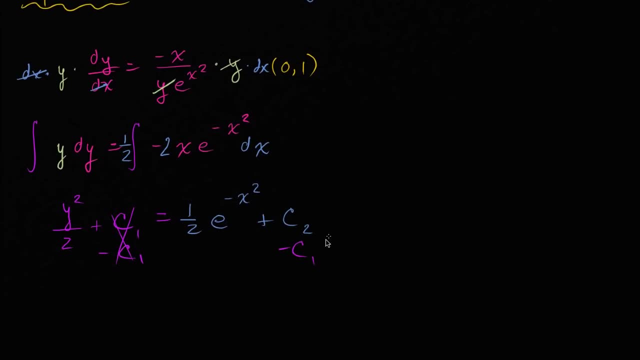 arbitrary constants. we don't know what they are yet, And so we could just rewrite this as on the left-hand side we have: y squared over two is equal to. on the right-hand side. I'll write one half e let me write that in blue. 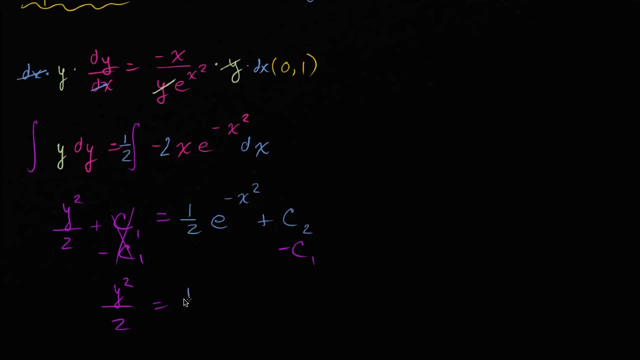 just because I wrote it in blue before: One half one half e to the negative x squared And I'll just say c two minus c one, let's just call that c. So if you take the sum of those two things, let's just call that c. 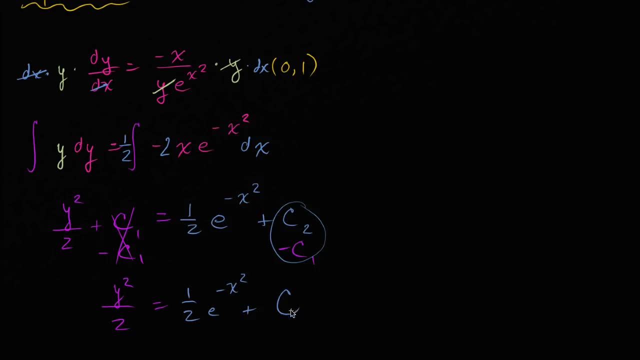 And so now this is kind of a general solution. We don't know what this constant is And we haven't explicitly solved for y yet, But even in this form we can now find a particular solution using this initial condition. Let me separate it out. this wasn't part. 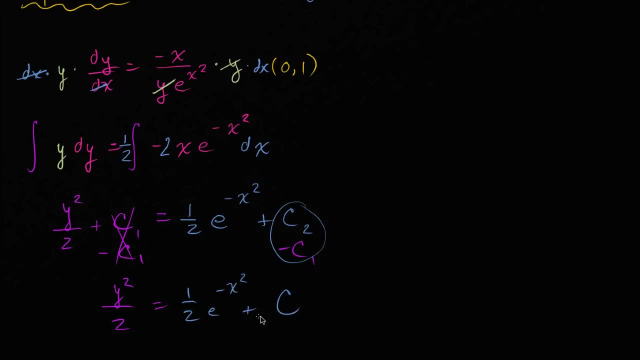 And we haven't explicitly solved for y yet. But even in this form we can now find a particular solution using this initial condition. Let me separate it out. This wasn't part of this original expression right over here, But using this initial condition. 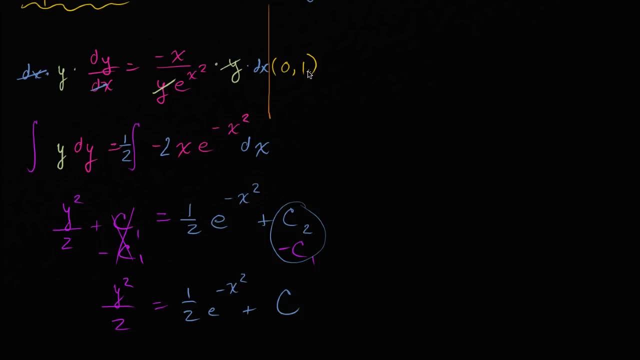 So it tells us, when x is zero, y needs to be equal to one. So we would have one squared which is just one. over two is equal to one half e to the negative zero squared. Well, that's just going to be: e to the zero is just one. 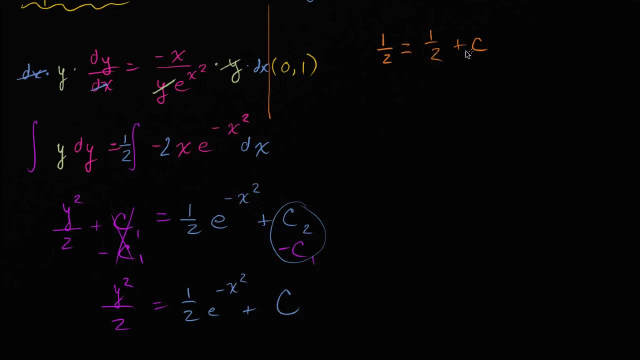 So it's going to be one half plus c And just like that we're able to figure out: if you subtract one half from both sides, c is equal to zero. So the relationship between y and x that goes through this point. 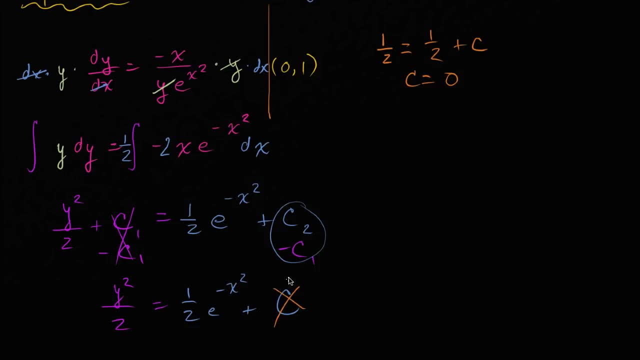 we could just set: c is equal to zero, So that's equal to zero. That's zero right over there. And so we are left with y squared over. two is equal to e, to the negative x squared over two. Now we can multiply both sides by two. 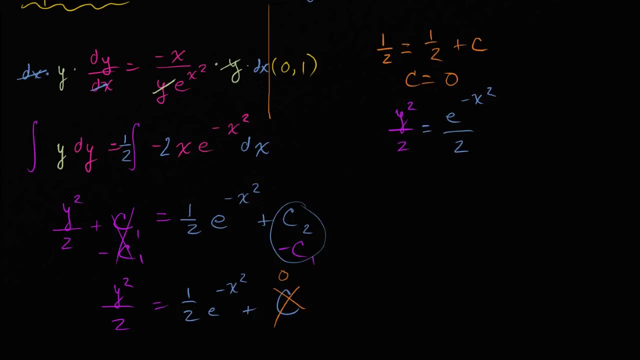 And we're going to get y squared, y squared, let me do that. So we're going to get y squared is equal to, is equal to e, to the negative x squared. Now we can take the square root of both sides and you could say: 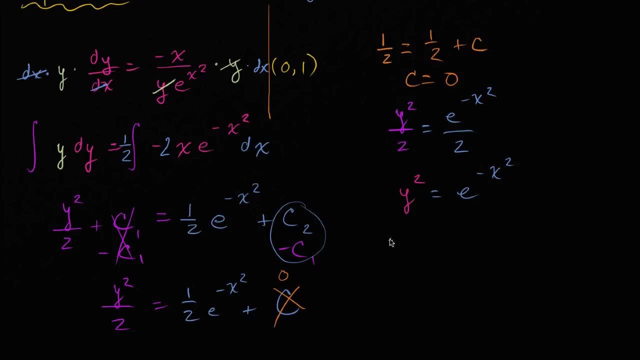 well, look, y squared is equal to this. So y could be equal to the plus or minus square root of e, to the negative x squared. But they gave us an initial condition where y is actually positive. So we're finding the particular solution. 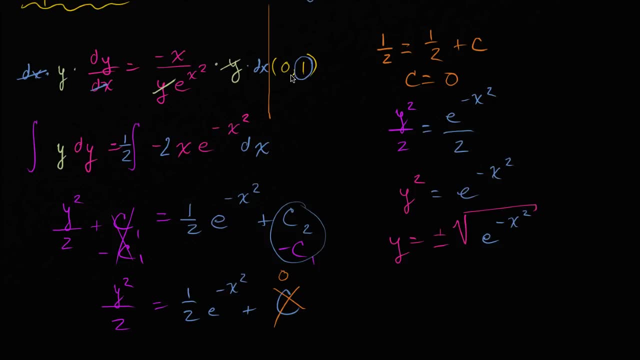 that goes through this point, That means y is going to be the positive square root. If this was the point zero negative one, then we would say y is the negative square root. But we know that y is the positive square root. It's the principal root right over there. 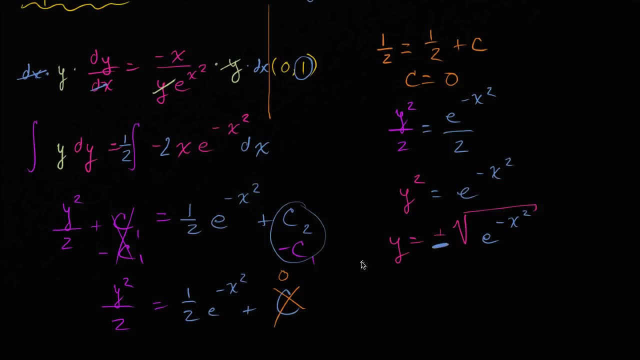 So let me do that a little bit neater So we can get rid of whoops. I thought I was writing in black, So we can get rid of this right over here. We're only going to be dealing with the positive square root. 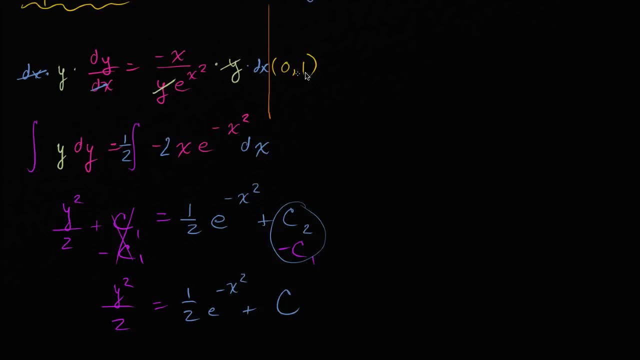 this wasn't part of this original expression right over here, But using this initial condition. So it tells us: when x is zero, y needs to be equal to one. So we would have one squared which is just one over two is equal to one half e to the negative zero. 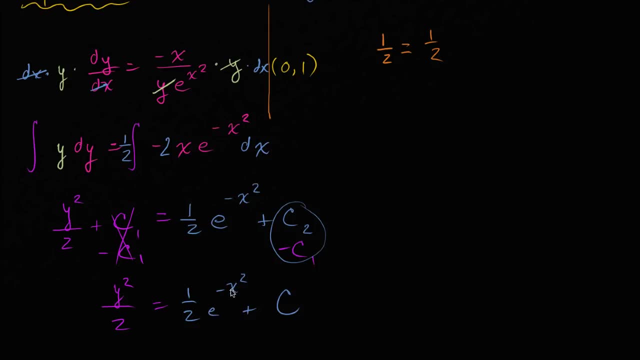 squared. well, that's just going to be e to the zero is just one, so it's going to be one half plus c, And just like that we're able to figure out: if you subtract one half from both sides, c is equal to zero. 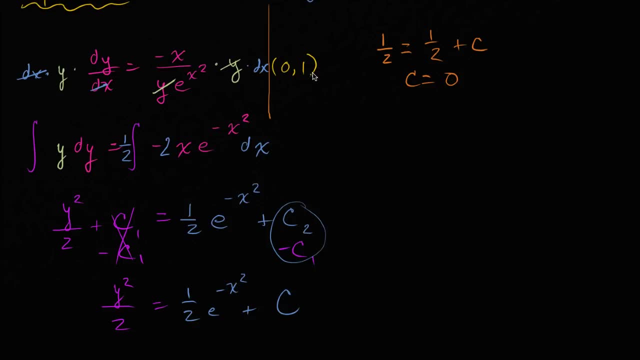 So the relationship between y and x that goes through this point we could just set: c is equal to zero, So that's equal to zero, that's zero right over there. And so we are left with y squared over two is equal to e, to the negative x squared over two. 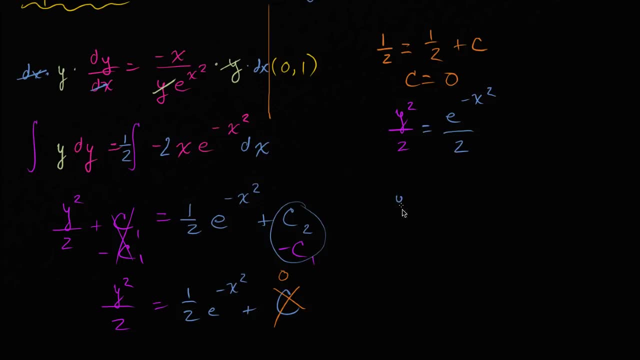 Now we can multiply both sides by two and we're going to get y squared. y squared- let me do that- So we're going to get y squared is equal to e, to the negative x squared. Now we can take the square root of both sides. 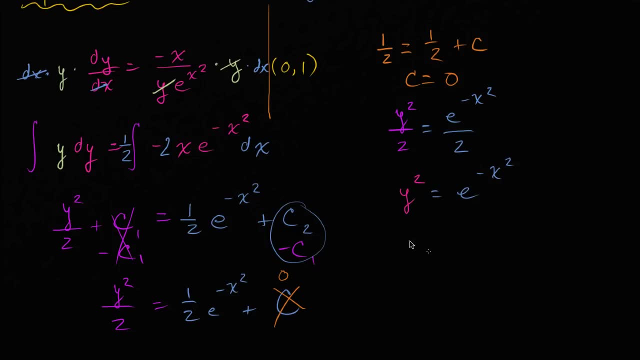 and you can say: well, look, y squared is equal to this. so y could be equal to the plus or minus square root of e to the negative x squared, of e to the negative x squared. But they gave us an initial condition. 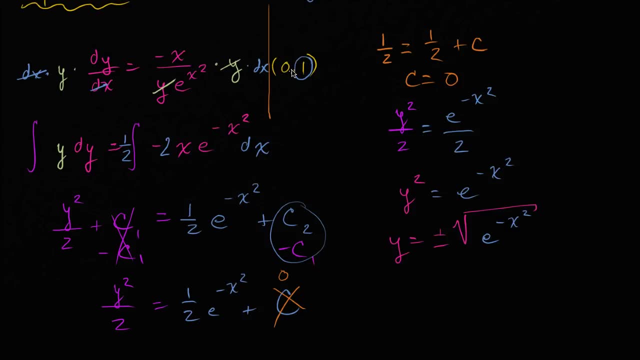 where y is actually positive. So we're finding the particular solution that goes through this point. That means y is going to be the positive square root. If this was the point zero- negative one, then we would say y is the negative square root. 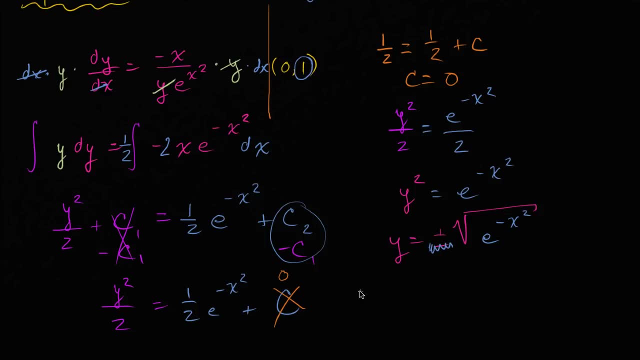 But we know that y is the positive square root. it's the principal root right over there. Actually, let me do that a little bit neater So we can get rid of whoops. I thought I was writing in black, So we can get rid of this right over here. 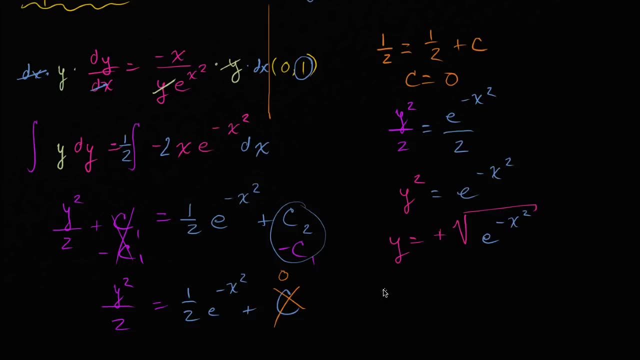 We're only going to be dealing with the positive square root, Or we could. so we could write: y is equal to e to the negative x squared to the 1 1⁄2 power, And that, of course, is equal to e to the negative x squared over two.